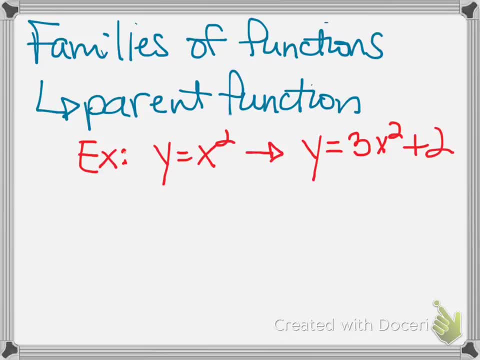 3x plus 2.. That would just be one member of the family of functions. led by that. parent of y equals x squared. There are lots of different types of parent functions. Y equals x cubed, The cubic function would be one. Y equals the square root of x. That's another type of function In the next. 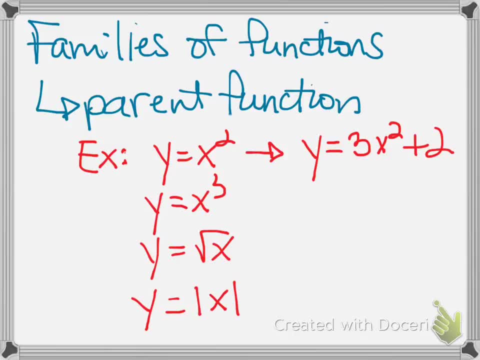 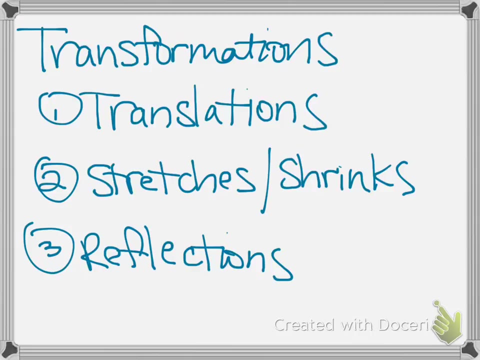 section we're going to talk about the function. y equals the absolute value of x. So those are just some of the examples of a parent function, but there are many, many more possibilities. So there are actually three different types of transformations. Again, in this video we're 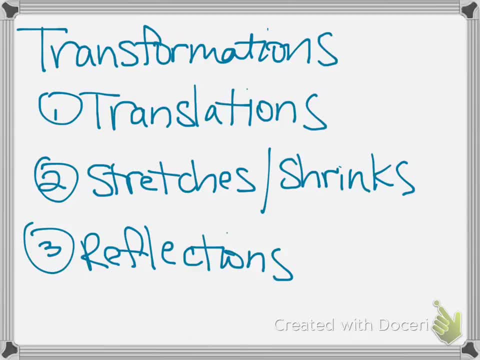 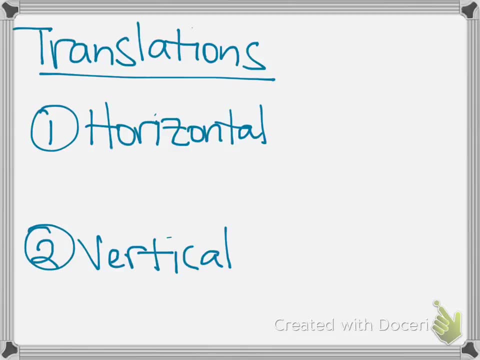 particularly interested in translations. In the next video we'll talk about stretches and shrinks and then, finally, we'll talk about reflections, But for now, let's focus on translations. There are two different types of translations, either horizontal or vertical, And, of course, if we have a horizontal translation, that means that we are moving our function to. 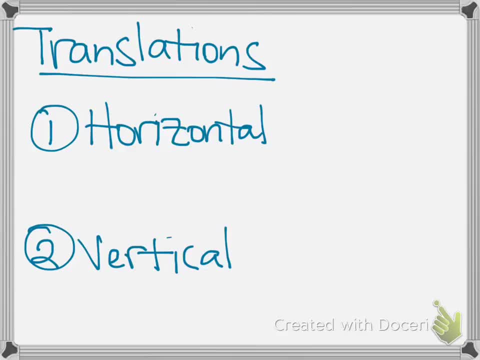 the left or to the right, And then we have a horizontal translation. that means that we are moving the function up or down. So, if you remember, back to section 2.1, we talked about function notation And that's going to come back here. So if we take our parent function and we apply what's, 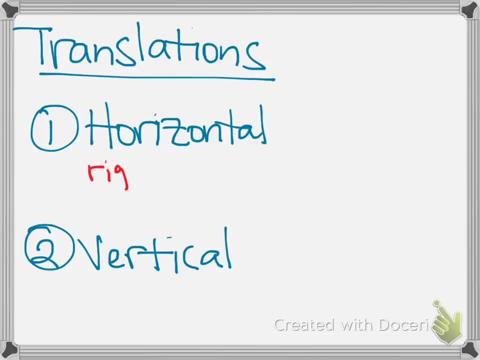 called a horizontal translation. Like I said, we can either move to the left or to the right. If we're moving to the right, that means I'm representing the translated function with y. That means that we are taking our original function, which was f of x and we are shifting it to. 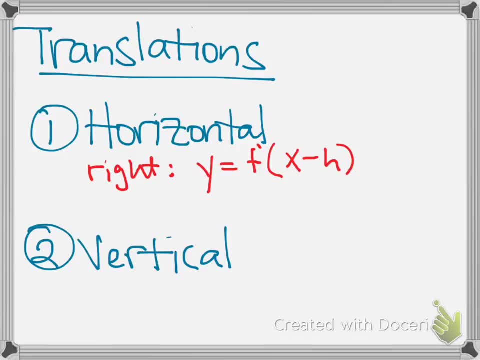 the right h units And so we represent that as f of x minus h. And conversely, if we are going to translate our parent function to the left, then our new function, y, would be the original function at h units to the left, and that's represented by x plus h. 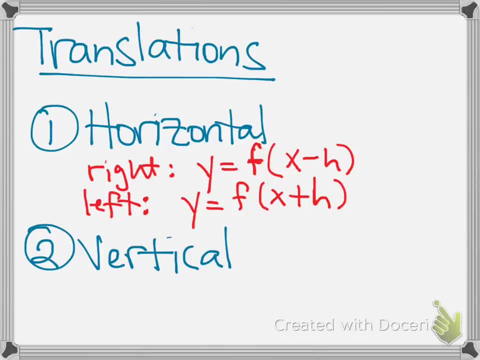 Now that might be a little bit confusing, because you do think normally that if I'm moving to the right, then shouldn't I be adding, and moving to the left means subtraction, And if you're working on the number line, that's certainly the case. 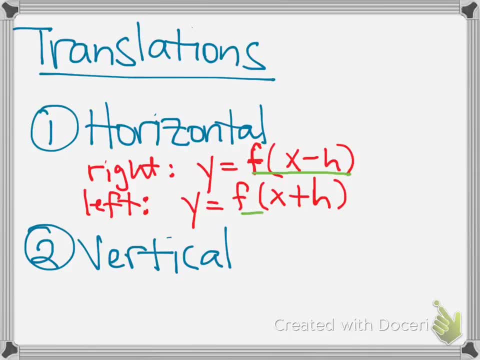 But just keep in mind that here, for these translations, it's actually the opposite of what you might expect, at least in terms of the horizontal translations, And that's because what this is saying is that we are taking our function, and if we're 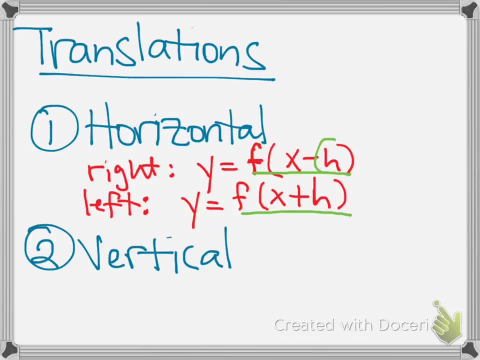 moving it to the right, then we would have to subtract h units to get back to our parent function. or if we took our parent function and moved it h units to the left, then we'd have to add those number of units back in to return back to our parent function. 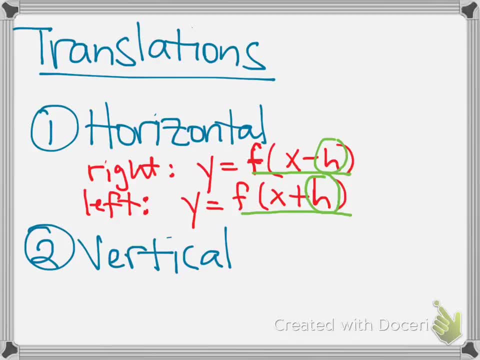 Now we also have. We have this idea of a vertical translation, and that works pretty much the same way as a horizontal does, except now we're moving up or down. If you're moving up a certain number of units, we usually talk about vertical translations. 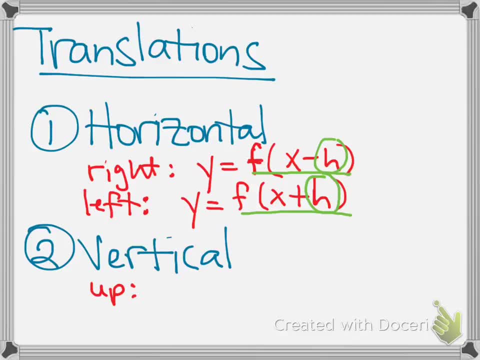 with the letter k- horizontal translations. you notice we use the letter h If we have a vertical translation and we're moving a certain number of units up. we can describe that by saying that y is going to equal f of x plus k. 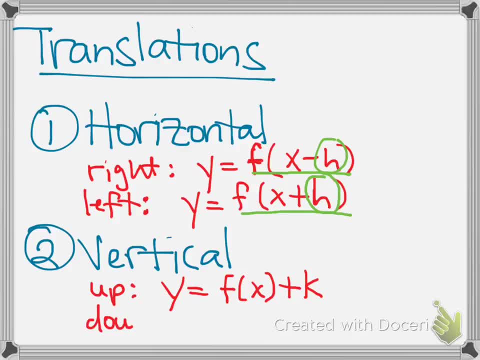 Meaning we move k units up, and if it's a vertical translation down, that means that y is equal to the original parent function f of x minus k. And again, this one's not quite as tricky to remember because the signs on k work about. 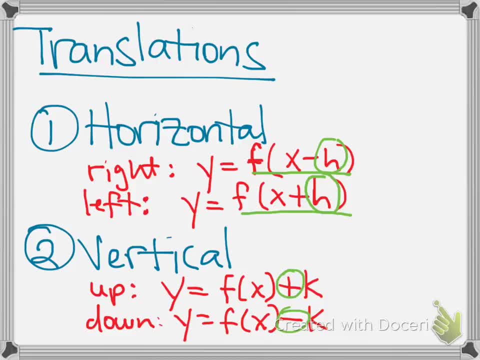 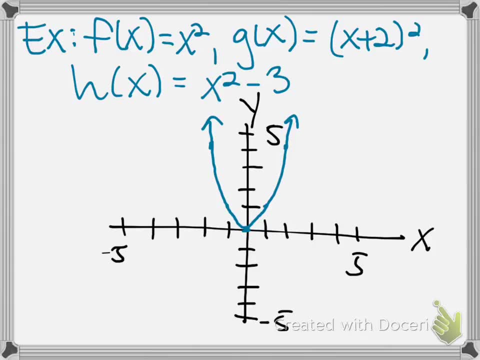 the same way as you'd expect. A positive value of k means you're moving up. a negative value of k means you're moving down. All right, So let's do a quick. Let's do a quick example Here. I have my parent function defined to be f of x equals x squared. 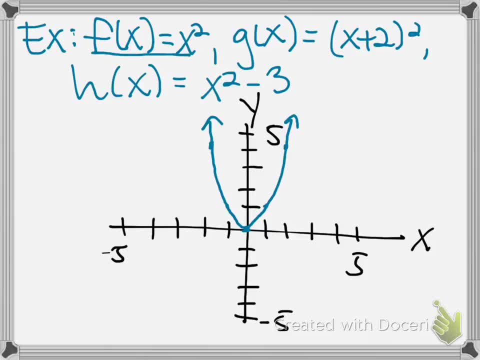 And that's just a regular old parabola. The vertex is at the origin. In my first translation I'm going to take our parent function f of x and I'm going to translate over to this new function g of x, where g of x equals x plus 2 squared. 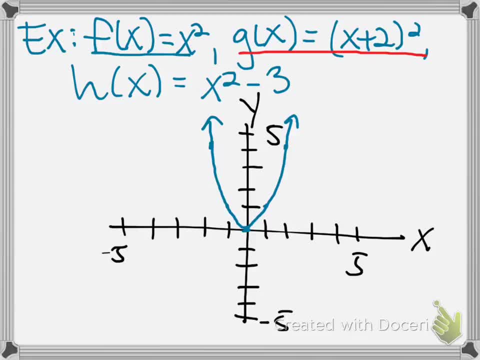 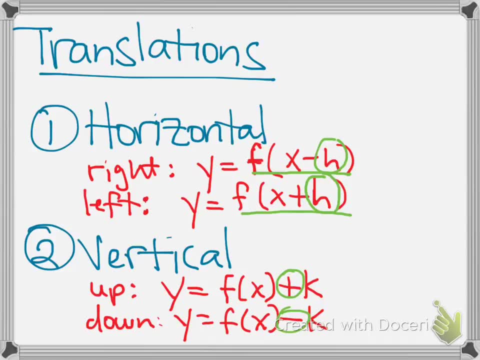 Now, if you think back to the last slide, we said that horizontal translation is going to be applied to the x-coordinate and vertical translations are going to get applied to the y-coordinate. So what we have here. let's see what I say: x plus 2 squared. so what we have, since we're